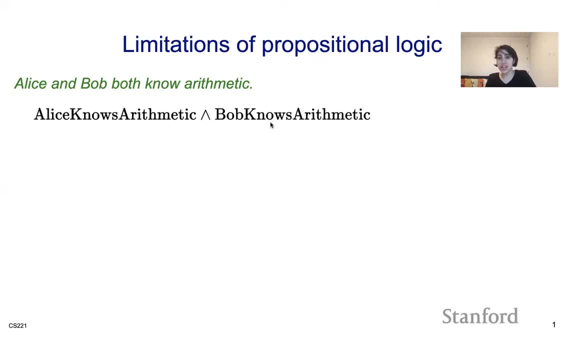 writing symbols and adding them and so on just doesn't scale. It's not expressive enough. Let's say I write: all students know arithmetic. If I'm writing all students know arithmetic, then I'm going to list all student names and then have a single propositional symbol for each of. 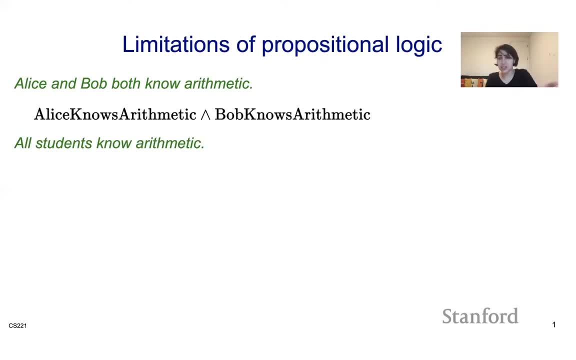 students knowing arithmetic and adding that And that just doesn't scale. If I have a lot of students, if you're in a class like 221, that wouldn't really scale right Like I need to write. Alice's student implies Alice knows arithmetic. Bob's student implies Bob knows arithmetic And. 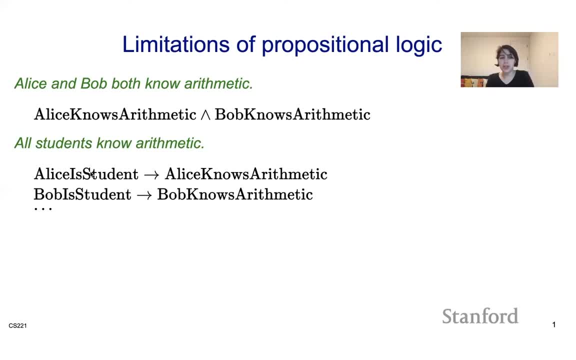 each one of these is going to be a symbol that takes like true, false by itself, And this is going to blow up fairly quickly. Even worse, like I can have a situation where I write a proposition that says: I write a statement that says every even integer greater than two is the sum of two primes. 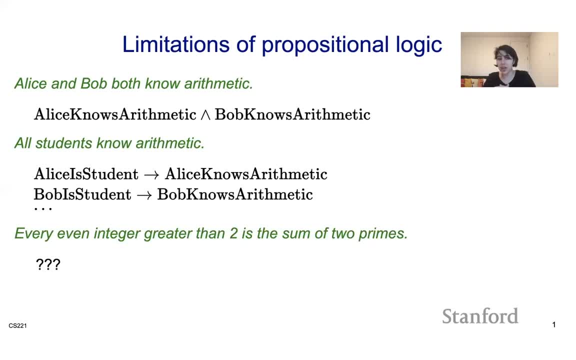 Okay, So this is actually a gold box conjecture. Okay, So if I want to write this in logic, well, I'm kind of screwed right, Like I can't write this in propositional logic because it's talking about every even integer and there's an infinite number of them. So I'm not going to be. 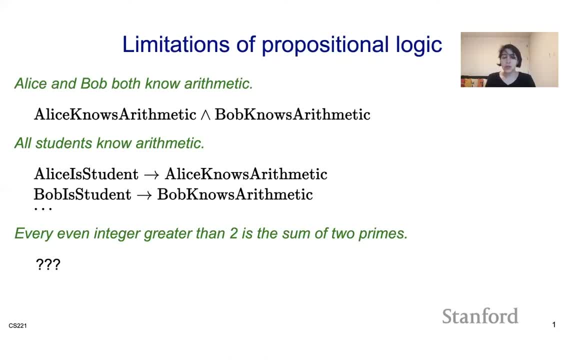 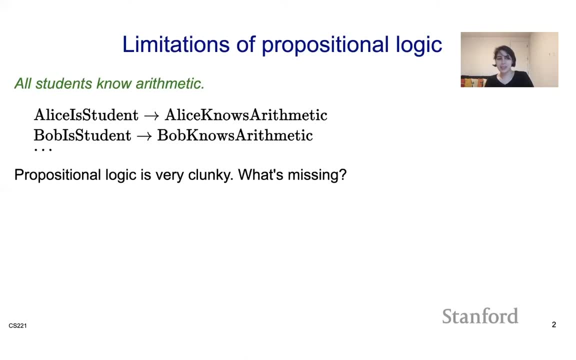 able to write that in propositional logic. Okay, So, so what can we do? It looks like if I'm using propositional logic, it's very clunky. And then there is: there is kind of like a lot of proposition, a lot of propositional symbols going on and it just 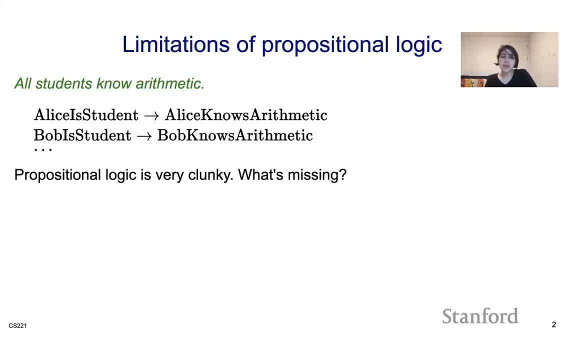 wouldn't scale. But if you think about it, like when you're thinking about these statements, there are some objects here and and some relationships, some predicates between these objects And maybe we can use that structure. There's quite a bit of structure here, right? 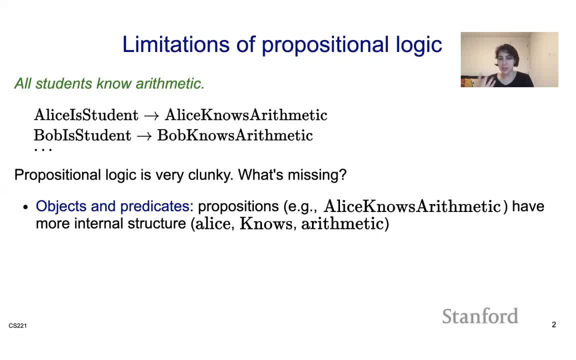 Like Alice being a student or Bob being a student. right, Like being a student is is a predicate on top of this object, object being Alice or object being Bob. Maybe we can use that structure And instead of defining a single propositional symbol for 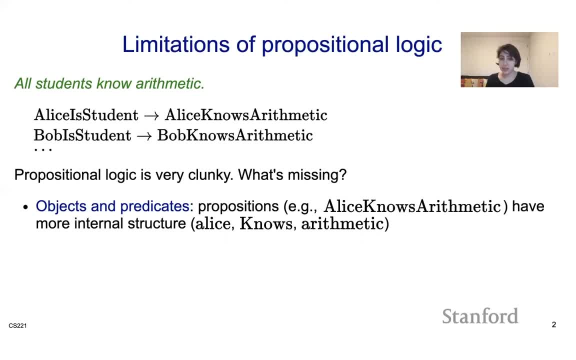 everything. maybe we can talk about objects and predicates instead. Okay, So so what that means is here, for example, like in this other example, Alice, knowing, arithmetic, Alice, you can think of it as an object, Arithmetic, you can think of it as an object, and knowing is a predicate on top of 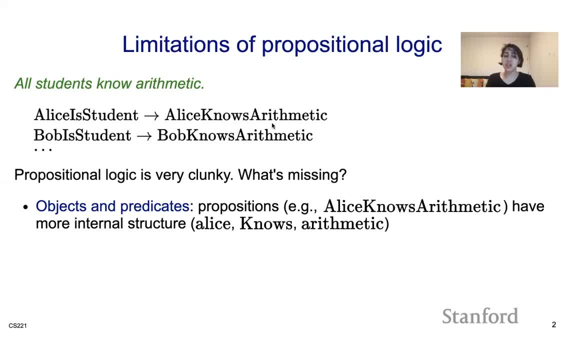 Alice and arithmetic And- and maybe we can, we can think about that structure And in general this other view that there are some objects and some predicates on top of them, and think of that as a way of writing a new type of logic In addition to that like for that. 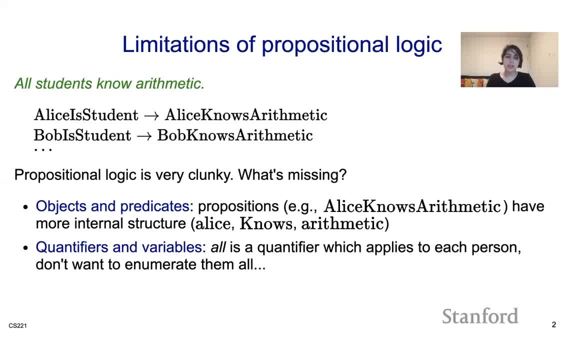 example, when I was talking about every integer having a property, then for, for those types of types of specifications, we need to think about quantifiers, right? We need to think about ways of saying for all, or ways of saying there exists So. so we need to have a way of representing these. 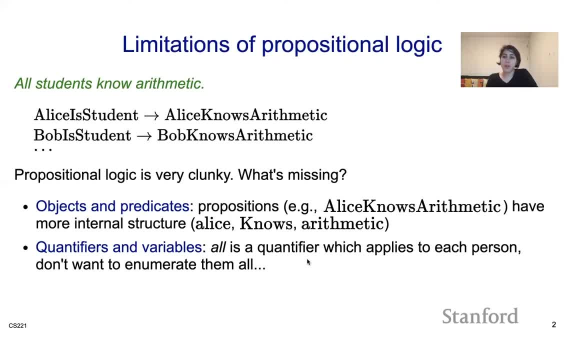 quantifiers. and to represent the quantifier, we need to have a variable right. So when I say for all students, right, I need to have a variable X that corresponds to every single student. So, in addition to these objects and predicates, we need to have quantifiers and variables, and then we need to use 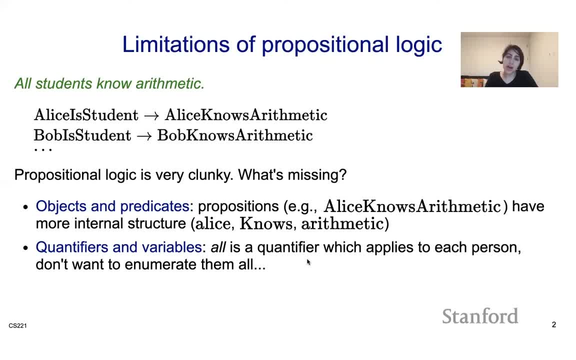 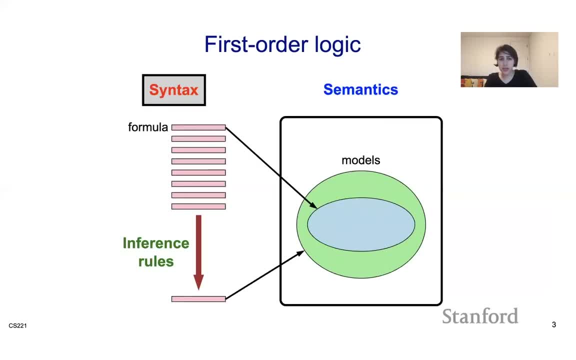 quantifiers and variables to represent, to represent our, our statements. Okay, Let me, let me give you an example. So, so what I want to do in this, in this module today, is I want to talk about the syntax of first order logic And I want to then talk about semantics of first order logic, And 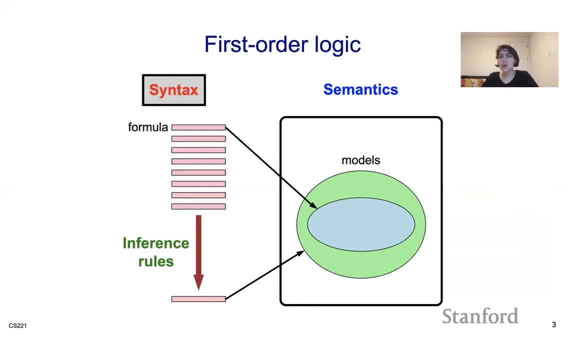 in the next module I'll be talking about inference rules, But I'm not going to go into as much like the. I'm not going to do justice here, So I'm not going to go into as much details in syntax and semantics, the same way that we did in propositional logic. 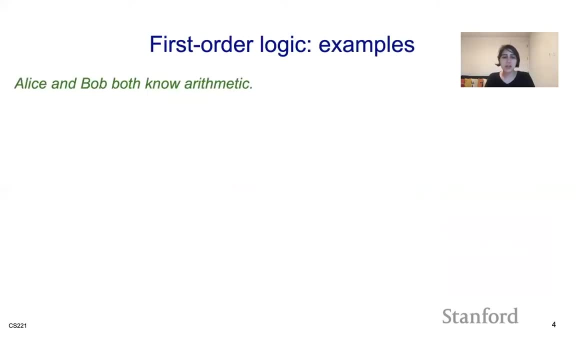 So it's a little bit more high level here, Okay, So so let me just give you a couple of examples here. So so, if I'm saying Alice and Bob both know arithmetic in first order logic, ideally I would want to be able to write something of this form, like something that says: Hey, 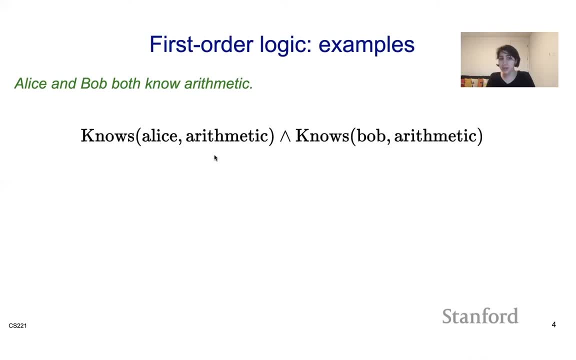 predicate of knowing over Alice and arithmetic, over these, these uh objects, Alice and arithmetic should be true, And the PR the same predicate of knowing over Bob and arithmetic. again, arithmetic is the same symbol, should be true. Okay So. 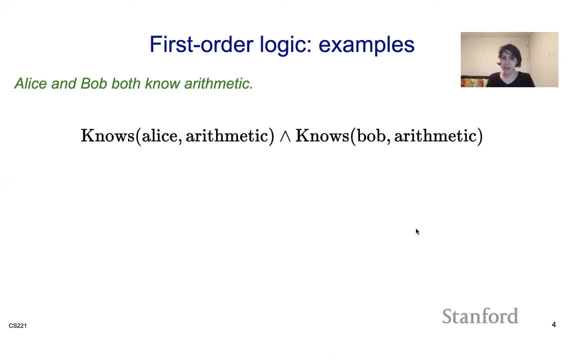 so I want to be able to capture that structure of objects and predicates in first order logic. The other thing is like going back to this other student, all students knowing arithmetic, I should be able to have quantifiers and variables. So so ideally, if I want to write this in first, 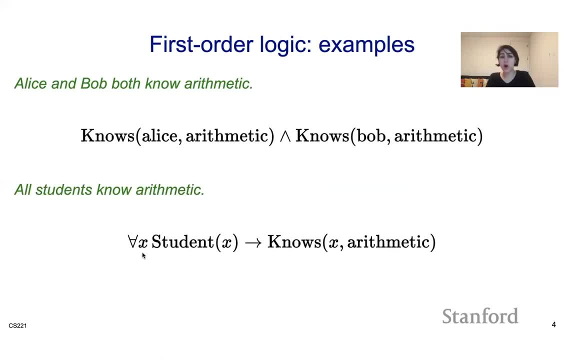 order logic: I w, I w. I should write something of this form For all: X. X being a student. predicate of student over variable of X should imply X, knowing your arithmetic. again, knowing is the same predicate. Okay, So these are actually just. 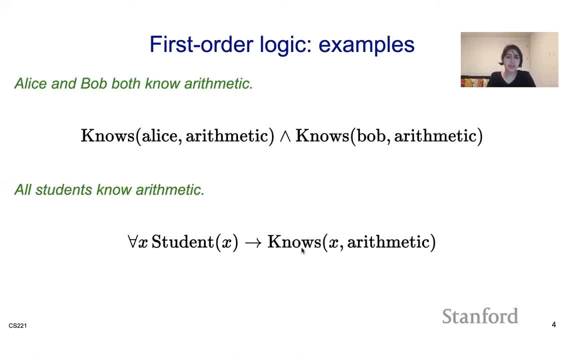 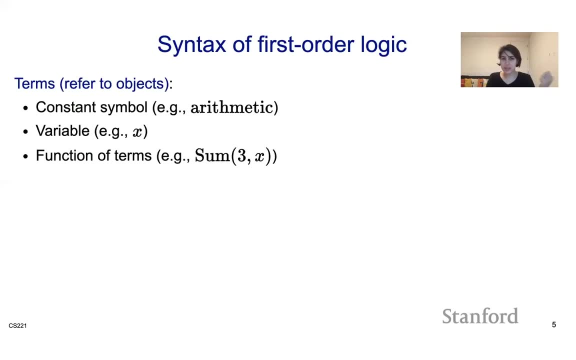 examples of first order logic. but but how do we do this? How do we get to these, get to these statements? for that We need to define the syntax of first order logic. So so let's get into the syntax of first order logic, All right, So let me go to my notebook. So, 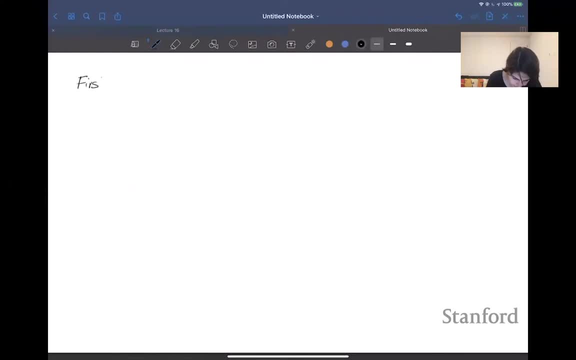 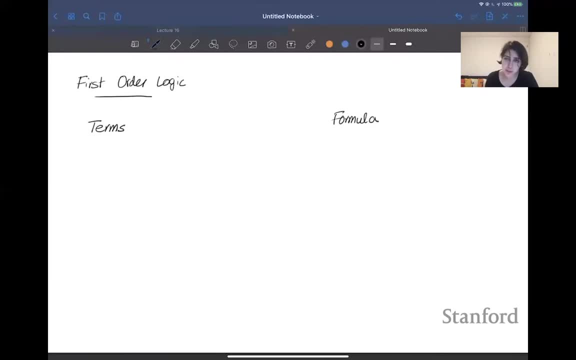 remember prepositional logic. we only had formulas here. Here, we first need to define a set of terms, and these terms are expressions that are referring to objects- Okay, So, so they are expressions that are referring to objects, Okay, Okay, So what are terms? So, so, the first thing. 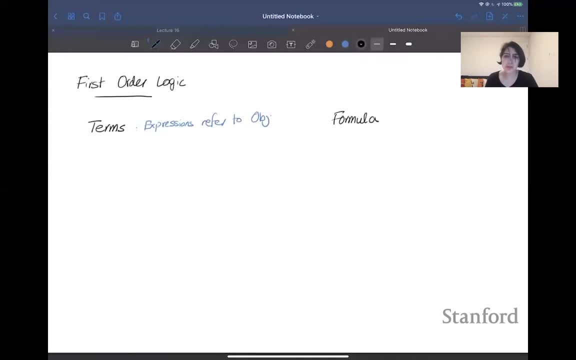 that we consider as term is a constant symbol. Okay, So Alice, for example, or mar else, or arithmetic, or whatever, These are constant symbols. Okay, So conscious symbol is is a term. Okay, Hmm, Yeah, Oh, sorry, Yeah, Hi back to. I didn't call it. this. this impossible, No problem. 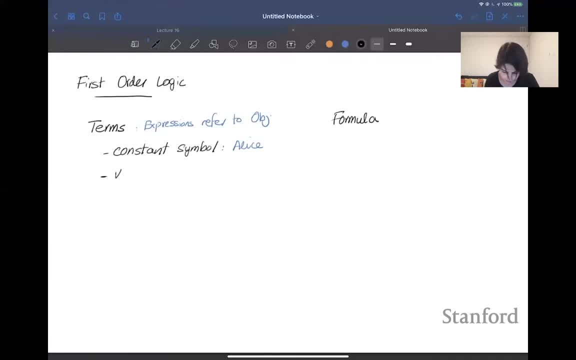 In addition to constant symbols, we need to have variables, like as I was talking about earlier. if you want to be able to talk about quantifiers, those quantifiers need to be defined over variables. So a variable is kind of like when I say for all, x, x does something, that x is a. 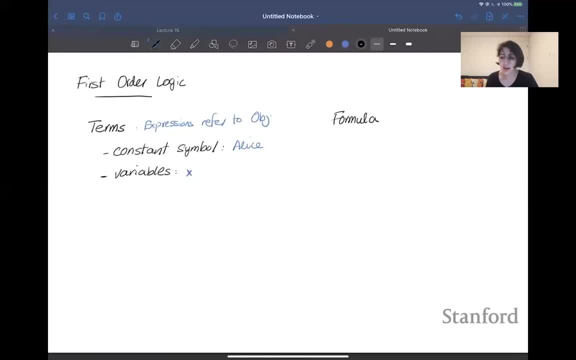 variable And in addition to that we can have functions here and these functions are defined on some of these terms. So functions can be defined on terms and they also give us terms. So, for example, I can look at a function like summing over x and 3.. So if I'm looking at sum of 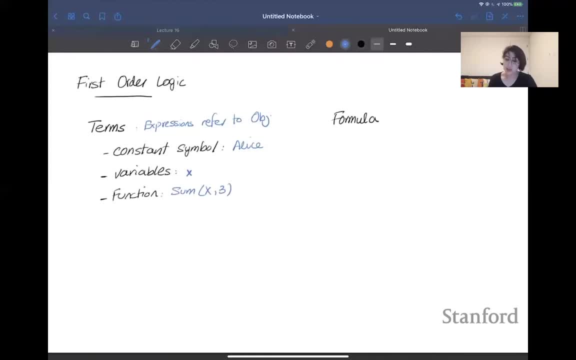 3 and x. x is a variable, 3, here is a constant symbol. summing over that is a function and that also gives me a term. All right, so that is terms. So now I can talk about formulas. So now, 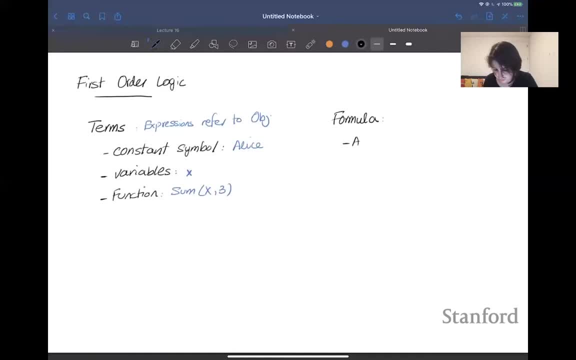 that I've defined terms, I can talk about formulas. The most basic form of a formula is an atomic formula. This is actually very similar to our propositional symbols in propositional logic, So this is kind of like the basis of it. right In propositional logic we had these propositional 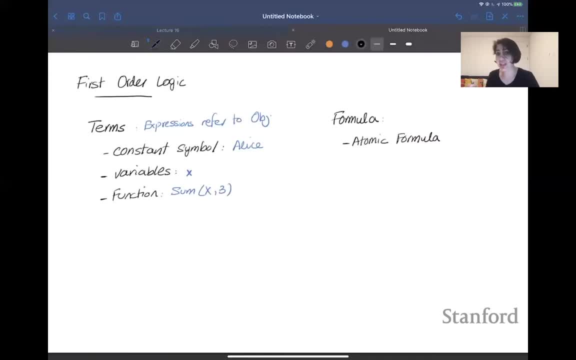 symbols like p or negation of p. We would define negation on top of that, but p was this propositional symbol. Here atomic formula is kind of like the basis of this logic. okay, So what is an atomic formula? An atomic formula is a predicate applied to terms. okay, So, for example, 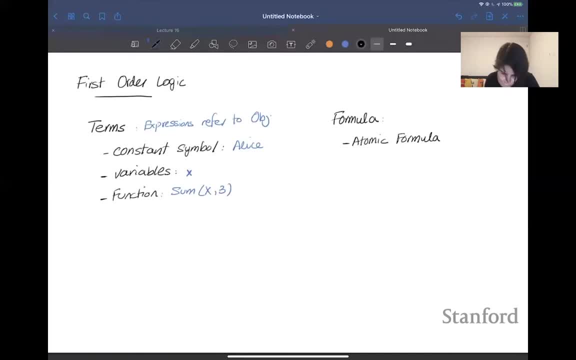 knowing the arithmetic is an atomic formula. I can write that, as knows, knows, is a predicate applied to symbol. constant symbol, Bob, and constant symbol arithmetic. okay, And this whole thing is an atomic formula. okay. So once we have the atomic formula, then what we can do is we can. 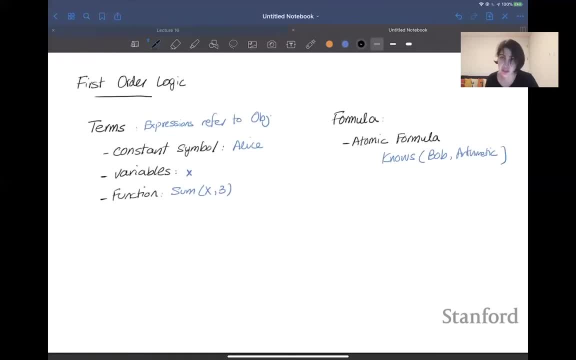 do operations on top of these, right, We could do the same things that we did in propositional logic, So we can write logical connectives on top of them, connectives on top of these, So applied to these formulas. so these logical connectives are things like negation, or or, or, and or implication. 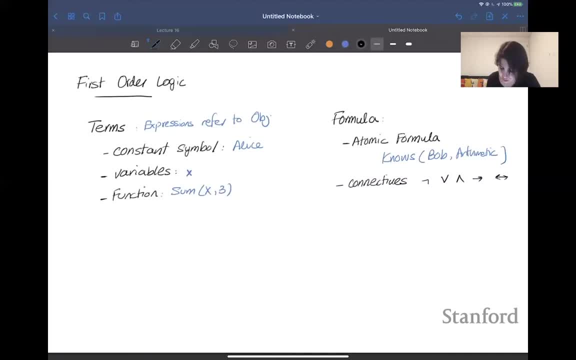 bidirectional implication. We can just apply the same sort of things similar to propositional logic here, And in addition to that we are going to define quantifiers. So quantifiers is going to be defined on top of all these, and these quantifiers are things like for all, for the 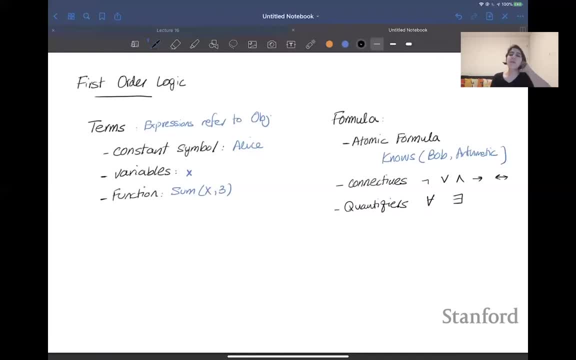 sum of x for the sum of y, for the sum of z. okay, All right. So this defines the syntax of our first order of logic. We have terms, we have formulas and then formulas. atomic formulas are basically going to be predicates on top of terms, And once we have the atomic formulas, we can play around. 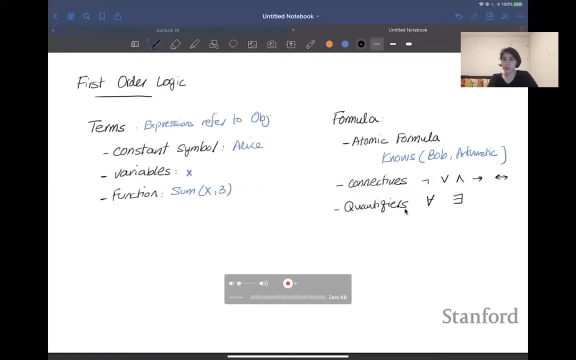 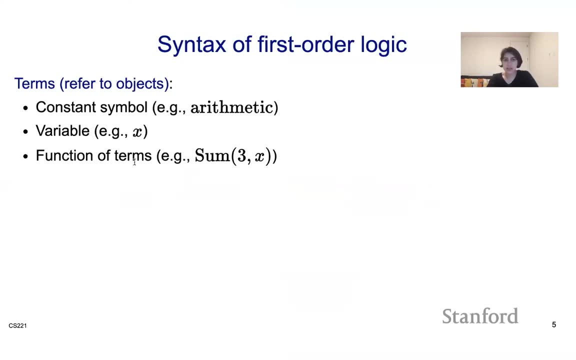 with them using the connectives, logical connectives or using the quantifiers. okay, Let's go back here. So a quick recap of that: constant symbols, like arithmetic variables, just like x functions, like sum of three and x, and then we have formulas referring to kind of like these truth values And atomic formulas. 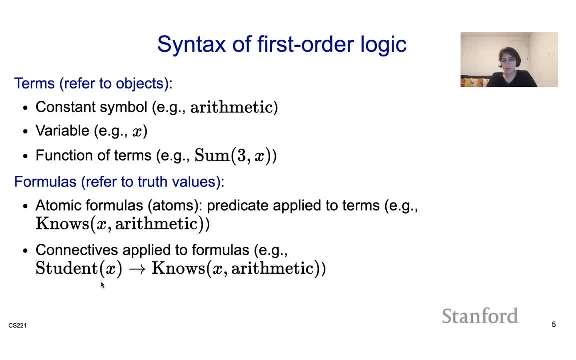 are predicates applied to terms, Connectives, connect them. For example, you might say: x is a student implies x knows arithmetic. So this implication is connecting this predicate on top of symbol, on top of the variable, to this predicate on top of the variable and the symbol. 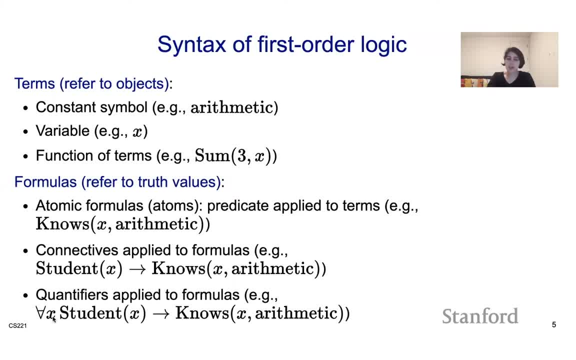 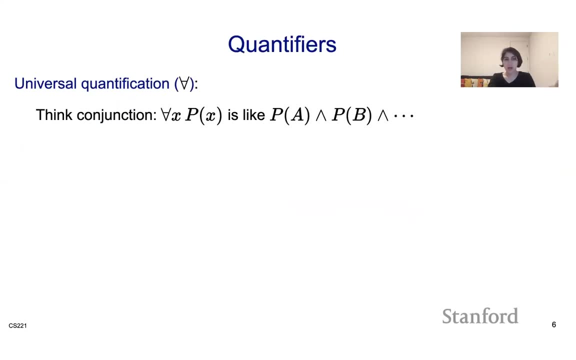 And then, in addition to that, once we have variables, we can have quantifiers. You can say: x is a student and that implies x knows arithmetic. okay, All right. So that summarizes the syntax of first order logic. One quick note on quantifiers is: if you think about quantifiers, quantifiers are. 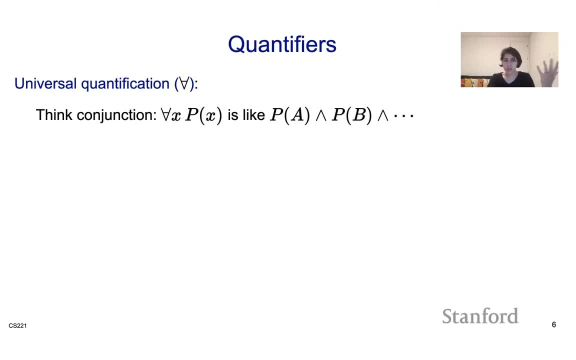 just slightly more complicated versions of ands and ors. So if you think about the for all quantifier, the universal quantification, you can think of it literally as a conjunction. okay, So when I say for all x, p of x, that's very similar to saying p of a and. 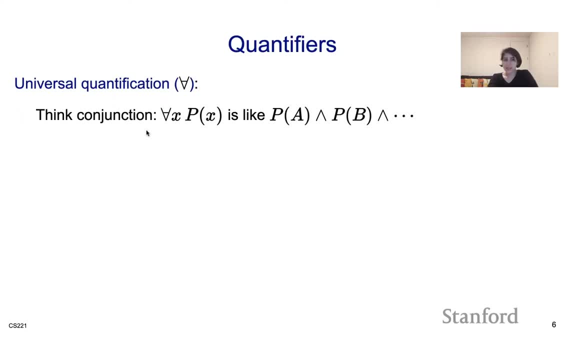 p of b and p of c and so on. okay, And this for all is kind of like being treated as ands between all the possible things that this x can take. okay. Similarly, if you talk about existential quantification, there exists that is kind of like an, or You can think of it as. 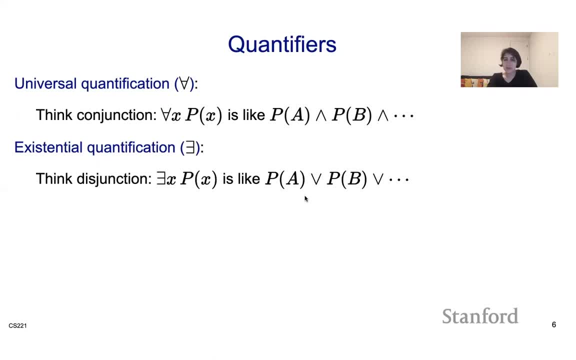 a disjunction. If I say there exists x, p of x, it's very similar to saying p of a or p of b or p of c and so on. okay, And if I have a finite number of them, then I can actually enumerate all of that. I. 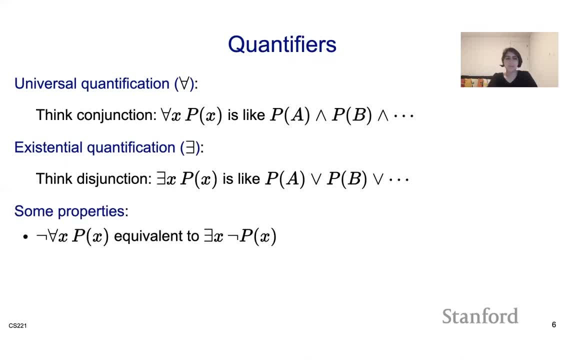 can actually unroll this and enumerate all of them, okay. Okay, so then if for all and there exists are kind of like and and, or, then i can apply the Morgan's Law. So what that means is, if i have a negation outside of one of these quantifiers, if i say negation of for all, x px. 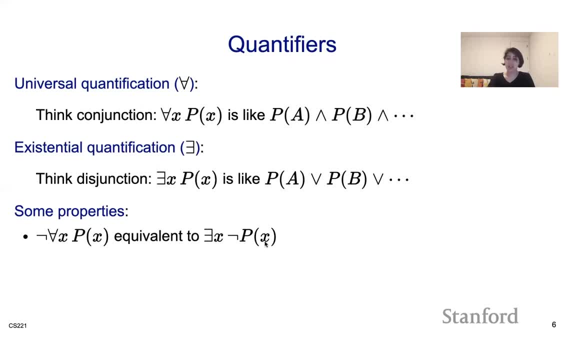 that is equivalent to saying: there exists x. negation of px. Why? Because the ands are going to be flipped to become ors, so for all becomes there exists and the negation becomes side, just like the Morgan's law applied to n's and o's. okay, All right. Another point I want to. 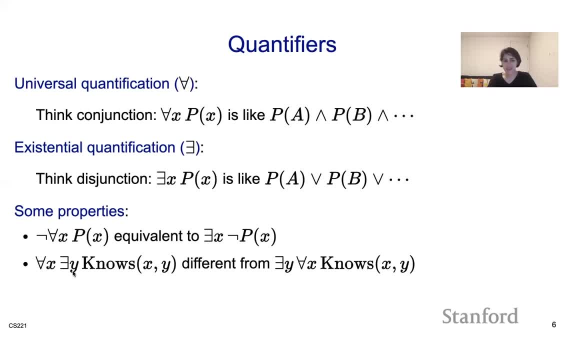 make here is if when you say for all x there exists y, we can't flip the order Again, just like n and o's, we can't really like flip this order, right If I say for all x there exists y, so then x knows. 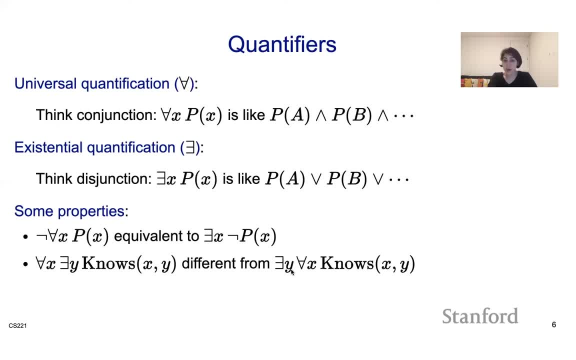 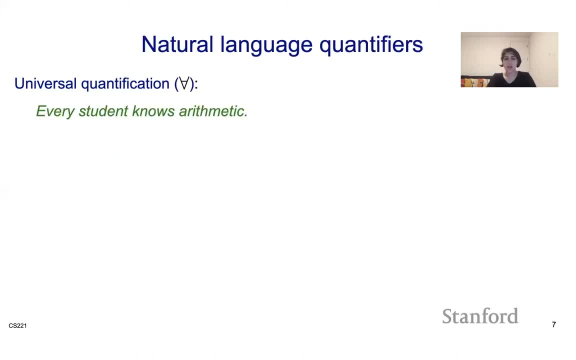 y. that's pretty different from saying there exists y such that for all x, x knows y, So we can't simply flip their orders. Do not do that, Okay. so now that we know the syntax of first-order logic, let's talk about how we can start from natural language and from natural language. 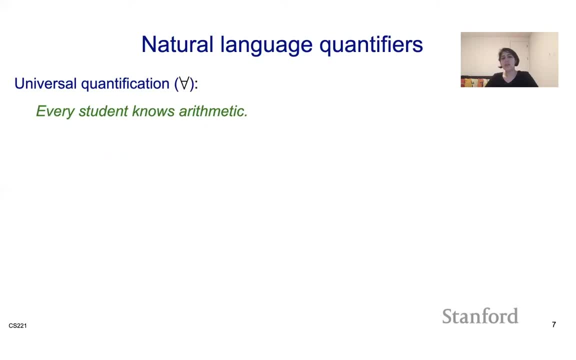 how can we write first-order logic? So if you think about universal quantification, when we talk about for all, the way that we usually refer to that in natural language is by using the word like every. okay. So if I say every student knows arithmetic, I would use the. 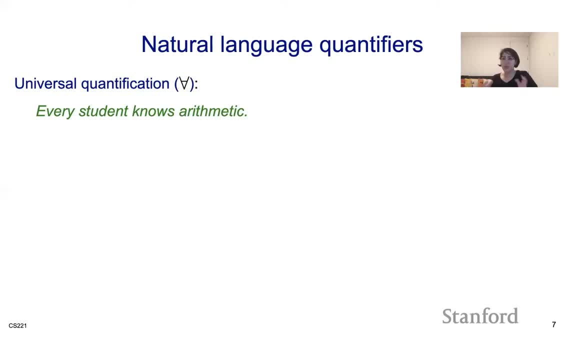 for all, like quantifier right, Like I would say for all x, because that corresponds to every student. So is this the right? so the question to ask is: is this the right way of writing this natural language statement? I have every student knows arithmetic. I would write for all x. 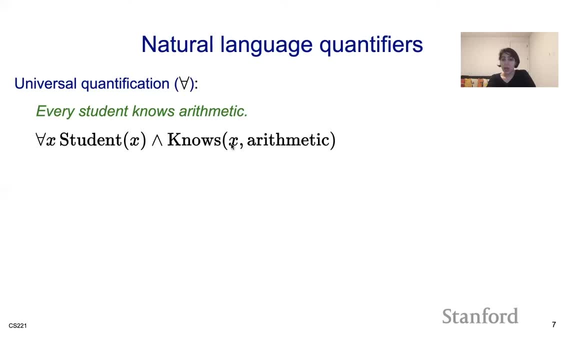 student x is student. okay, And then in addition to that I write: x knows arithmetic. But this doesn't actually correspond to this sentence, So there is something a little bit subtle going on here. Then you say: every student knows arithmetic. 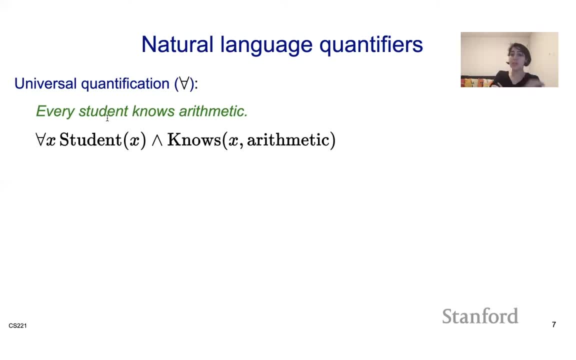 Basically, we are conditioning it like knowing arithmetic on being a student, But the statement here is not doing that conditioning. This statement is basically saying everyone is student and everyone knows arithmetic, And then that's not right. right, Not everyone knows arithmetic. 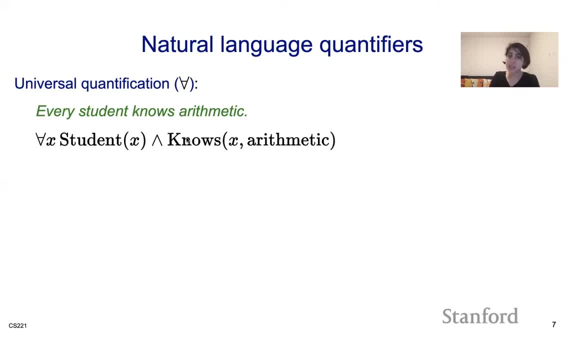 Every student knows arithmetic. So because there is that conditioning that goes on in our like in this statement and it's kind of like implied in this natural language, the correct way to write it is to write it in the natural language. So if I say every student knows, 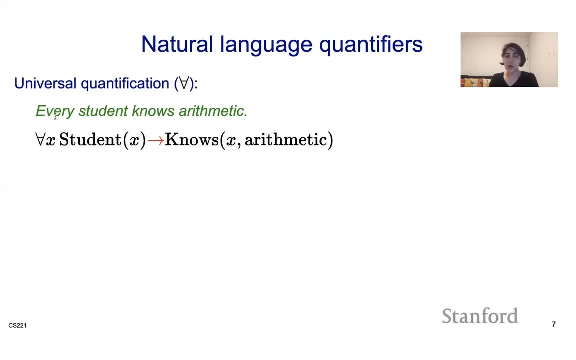 arithmetic. the correct way of writing this is by using an implication. So if I want to write out this statement- every student knows arithmetic, I would write for all x. if x is student, then that implies that x knows arithmetic. okay, So condition on that person being a student. 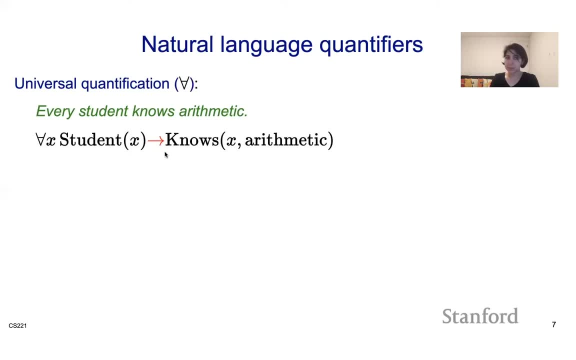 then x knows arithmetic And then that is an implication. We're going to have a couple of these examples in the assignment, the logic assignment. So I think it's kind of like a good rule of thumb to think about for all students. So I'm going to write for all x, if x is a student. 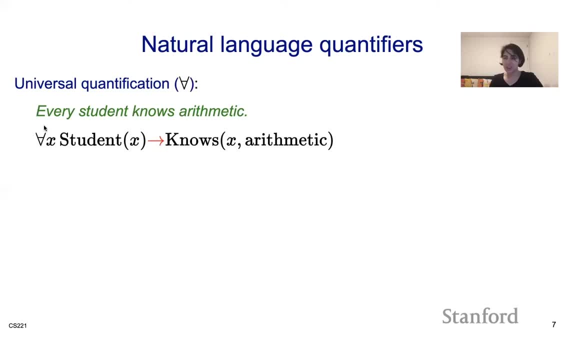 implies every time. you see every. So this is not always true, but in general, if you see, like every student or every person does whatever, it's usually of the form of for all implication. okay, How about there exists. So let's say that we have some student knows arithmetic. So when we talk, 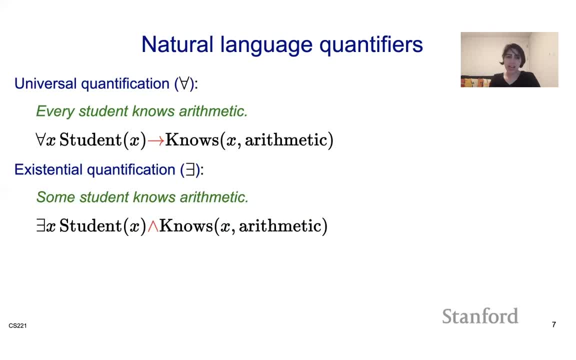 about some student, then we have to use existential quantifier, And the actual correct way of writing this is to say: well, there exists some student and x knows arithmetic. So when we talk about some student and x knows arithmetic, so an and is going to be sufficient here. So every time you 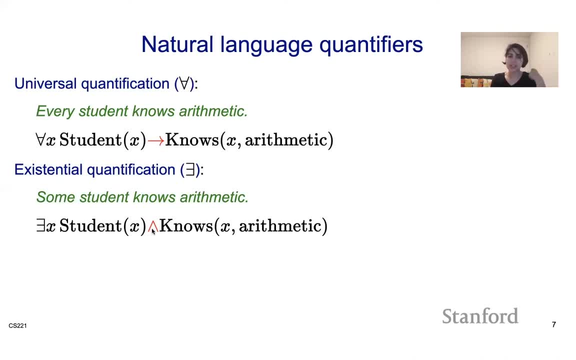 see a sum, it's usually corresponding to: there exists and an and And. every time you see every, it's usually corresponding to for all and an implication: okay, All right. So note that there are different connectives here. for all and there exists, usually when you start from natural. 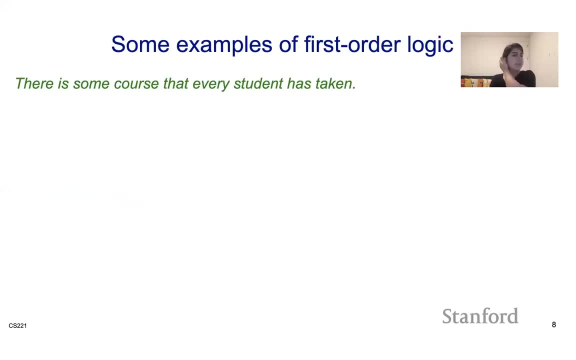 language. Okay, let's look at a few examples. Let's see examples. Let's see if we can write these in for all. Let's see if we can write these in for all. Let's see if we can write these in for a sort of logic. So first example is: there is some course that every student has taken. 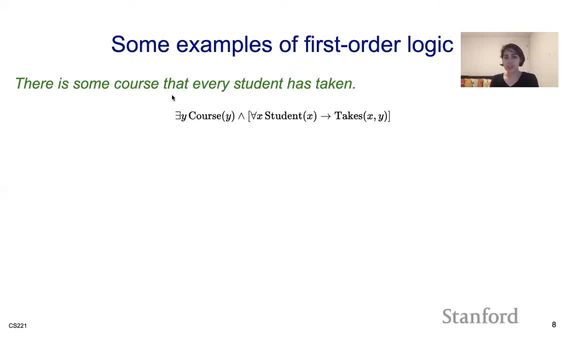 Okay, how do we write this? So there is some course, So there exists a y, such that y is a course. Okay, there is some course. This is to that part of it. There is some course, There is a y, So y is a course that every student has taken it. So that's the and part, And there is. 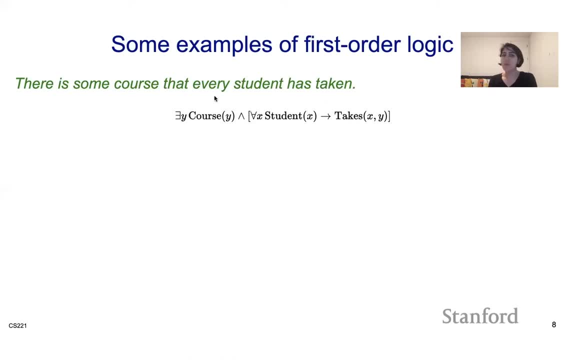 something true about this course. What is true about this course? Every student has taken it. So how do we write: every student has taken it. What that says is: for all x and x is a student, that implies that x- that student, has taken the course. y. Okay, All right, So that's the first. 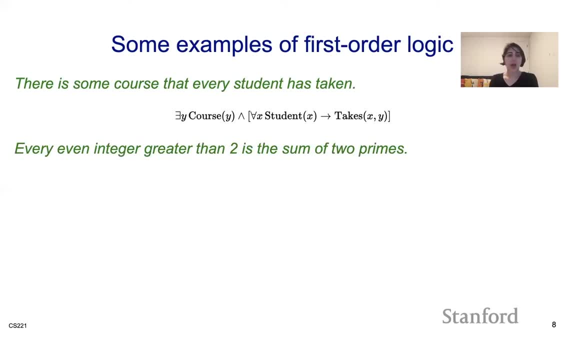 example. Let's look at the second example. So every- if you've seen this example earlier in this module. so every even integer greater than two is the sum of two primes. How do we write this So it says every even integer. So if it says: 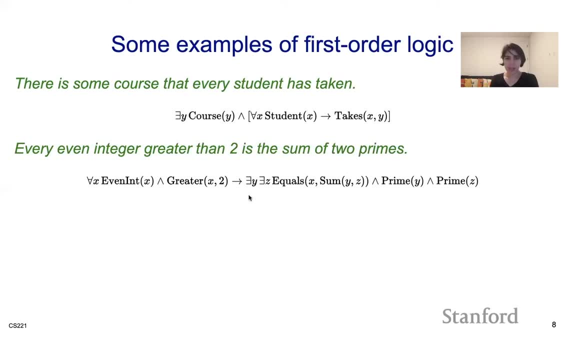 every. if I see every, then I would expect to see a for all x and some implication that comes later. So what is that x For all x? that x is an even integer, and this is greater than two. So for every, even integer, greater than two, So even integer, greater than two. What do I get for that? 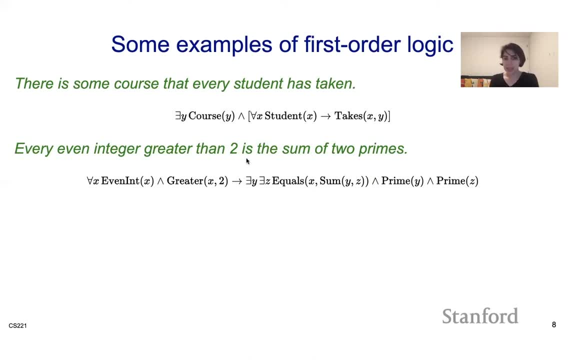 Even integer greater than two. That implies that that integer is going to be the sum of two primes. So how do I write that? I'm going to use there exists y and there exists c to correspond to those two primes, right? So so that integer is going to be sum of two primes. There exists a. 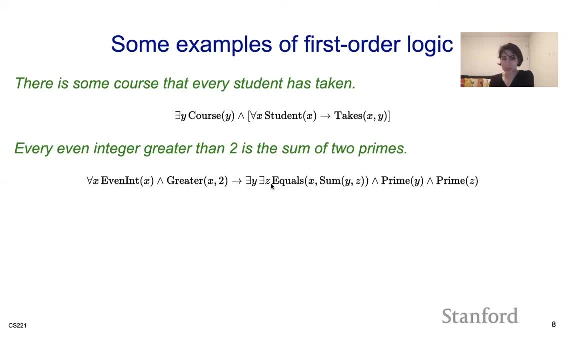 prime and there exists another prime, There exists a y and there is another z, So so that I I can say sum and y is a prime and z is a prime, and sum of y and z is equal to x. that integer, Okay, All. 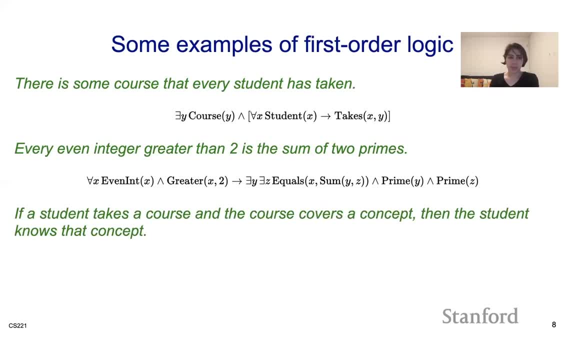 right. Okay, Let's look at another example. If a student takes a course and the course covers a concept, then the student takes a course and the course covers a concept, Then the student takes a course and the course covers a concept, Then the student knows the concept. So if it's kind of like 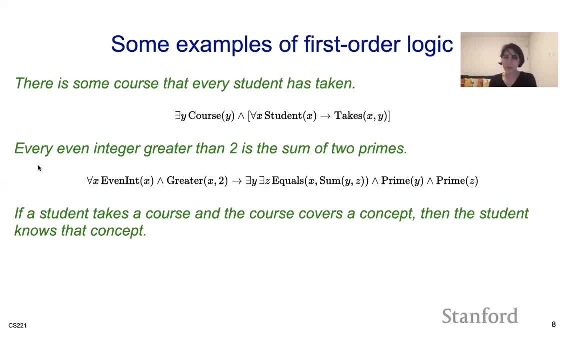 every. remember like every was also kind of like if right, Like when we were seeing every, we would say for all implies, If it's kind of the same thing, if it's basically saying, hey, if a student basically means for every student. So so if a student takes a course and the course covers a, 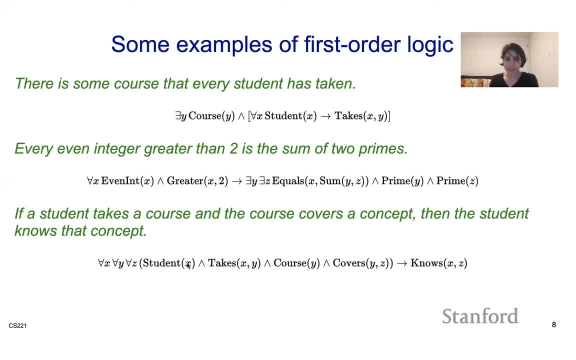 concept. then the student knows the concept. So for all x, x being a student. okay, And x takes a course y, So for all course y. then the student knows the concept. So for all x, x being a student. 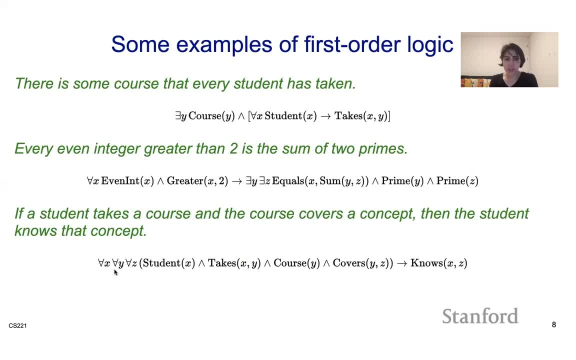 then the student knows the concept. So for all x. x being a student, then the student knows the concept. So so these four alls are for all students and for all course and for all concept. X is a student and x takes y and y is a course and y covers z. If you want it to be like pedantic and right, we should. 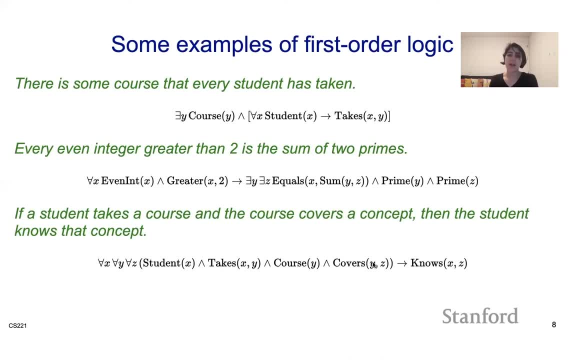 have had and z is a concept, but I'm skipping that. Then what does that tell me? Then the student knows the concept, right? The thing that comes after a comma is the thing that comes after, after this implication, right? Then the student x. 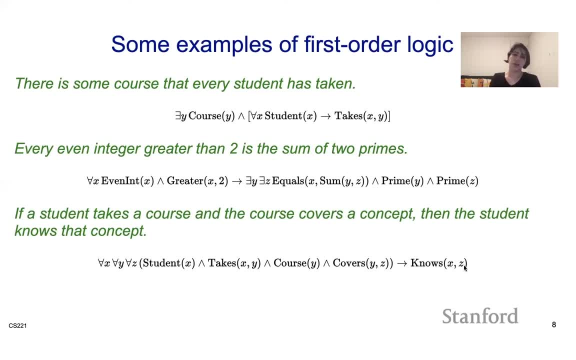 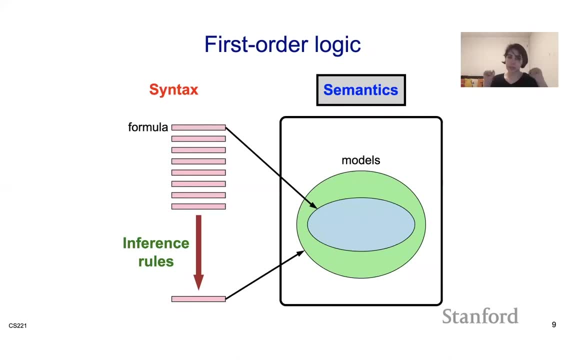 knows the concept. Okay, All right. So that was going from natural language to first-order logic, and we're able to talk about the syntax of first-order logic using terms and then using these formulas defined over terms. So now let's talk about the semantics of first-order logic. 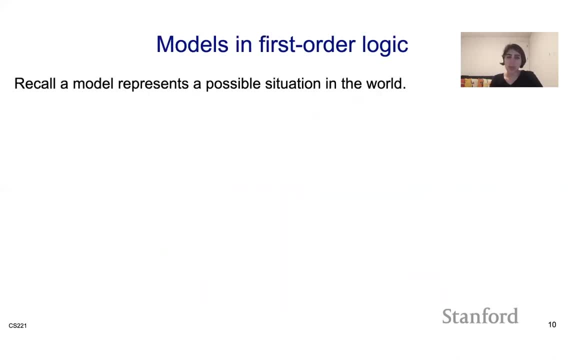 How do we define the meaning or semantics for this first-order logic? So, if you remember the semantics, how do we define semantics for propositional logic? We defined it by using this idea of models, right Like models representing a particular situation in the world. 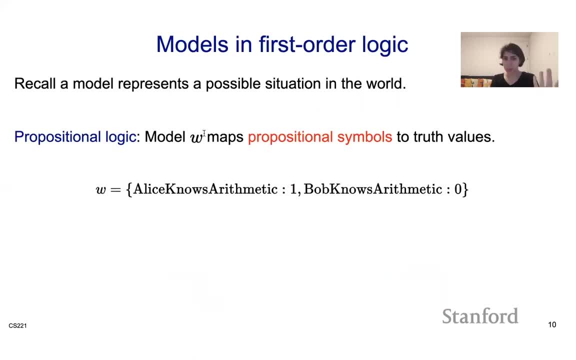 Okay, So in propositional logic a model W was a world that was mapping propositional symbols to truth values. It was a truth assignment to propositional symbols. So if, going back to my original example, Alice knows arithmetic and Bob knows arithmetic, if I were to write that in: 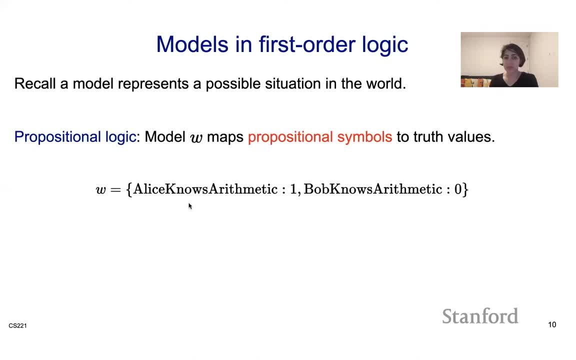 propositional logic. I would basically have these propositional symbols: Alice knows arithmetic, Bob knows arithmetic And in model would assign 1 or 0 to each one of these propositional symbols. That was in propositional logic. How do we think about it in first-order logic? 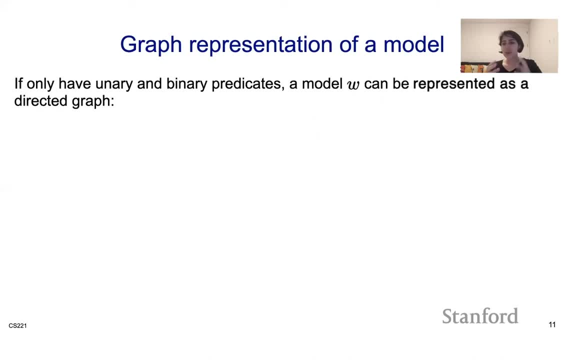 So the way we think about this in first-order logic is by having a graph representation for every model. So you can think about predicates that we have been talking about, like knowing, arithmetic and so on, as either unary or binary predicates that are defined over these terms that we are talking about. 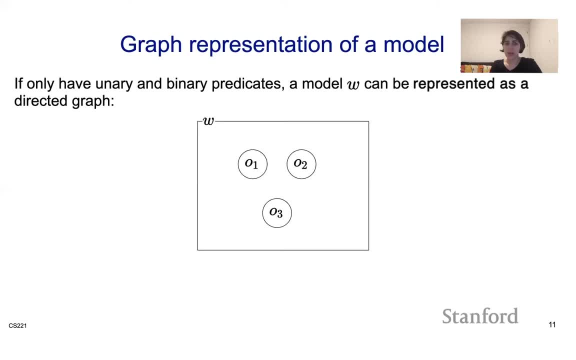 So a model w can basically be represented by a graph here. So a w could be a graph, where we have these different nodes And each node corresponds to an object. So an object is going to be represented by a node, And then we are labeling each node by a constant symbol. 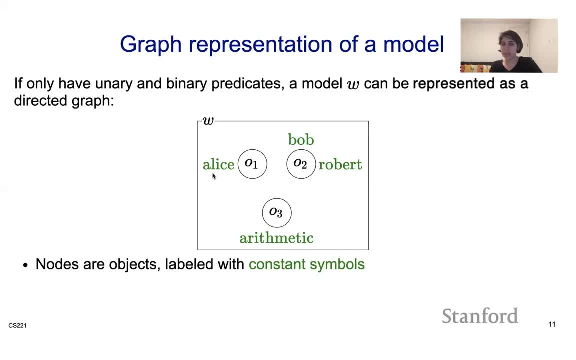 So node 1, O1 is an object and it's going to be labeled by Alice, And node 2 might be an object and it's corresponding to both Bob and Robert, And O3 might be an object and it's. 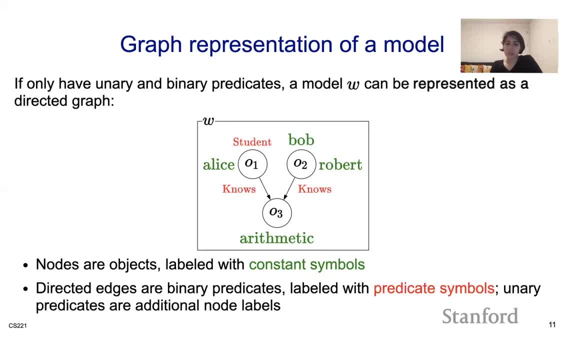 corresponding to a node, corresponding to an object, corresponding to an arithmetic, Then what we can do is we can have directed edges here that basically talk about binary predicates. So Alice, knowing arithmetic corresponds to this directed edge, that corresponds to this predicate, nodes applied to Alice, and Alice and arithmetic. 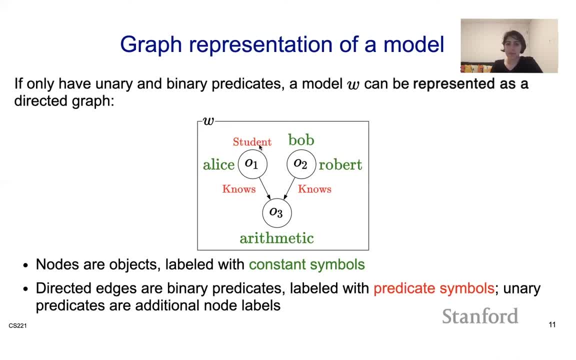 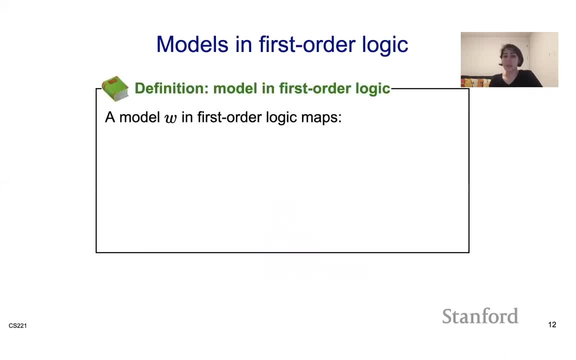 And for unary predicates. we are basically just going to have the predicate on top of the node. so Alice being a student, All right. so that defines a model here. So a model in the first-order logic basically has two components. One is that it basically has constant symbols assigned. 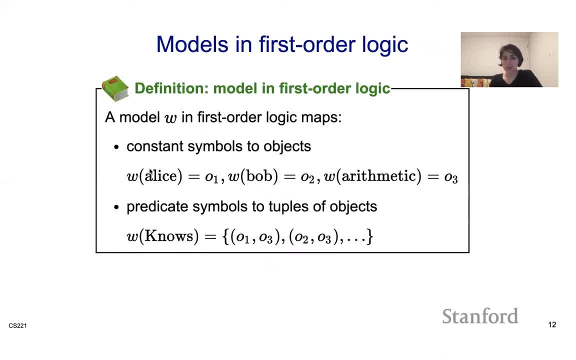 to objects. So basically, a model for Alice corresponds to a node O1, and Bob corresponds to node O2, and arithmetic corresponds to node O3.. And then we have predicate symbols that are basically giving us these two poles of O1, knowing. 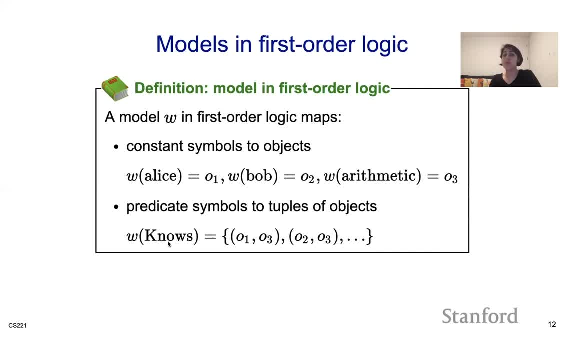 O3 or O2, knowing O3.. So that corresponds to W of knowing, that predicate of knowing, which basically gives us these two poles. Either they could be binary or unary, depending on the predicate. All right, so the way we are defining a model, 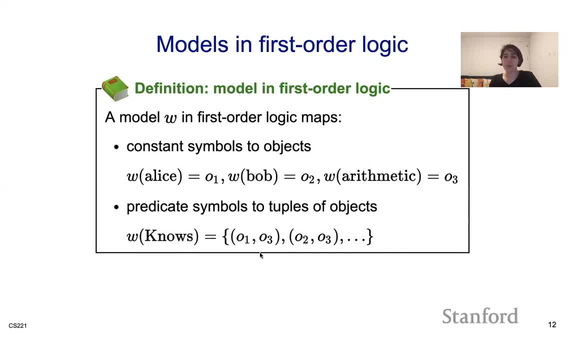 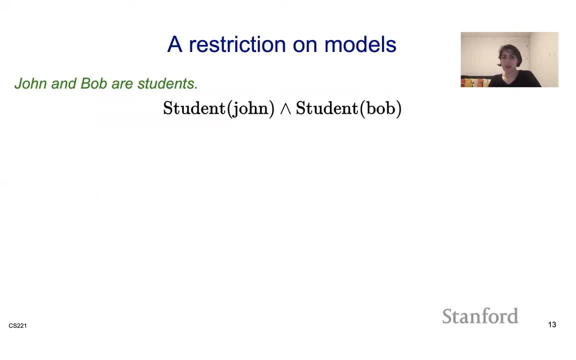 is a little bit more complex than the way we define model in propositional logic. So there are a few other restrictions that we are putting on models to make our lives a little bit easier. So, if you remember, OK, so we can have. basically. 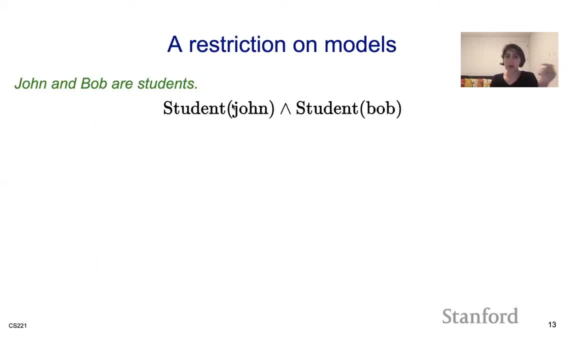 a statement that says John and Bob are students, right? So how do I write this? in first-order logic, I can say: John is student and Bob is student, So students are predicate on top of John and Bob. So if I think about a model corresponding to that, 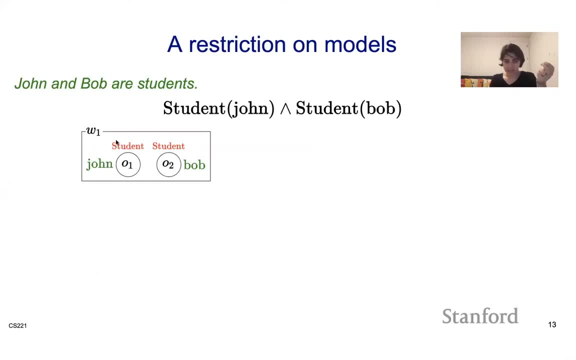 I can have a node O1 corresponding to John and predicate student on top of this node, and I can have node O2 responding to Bob and student on top of this. But that's one option, right. One could have other types of models that represent this. 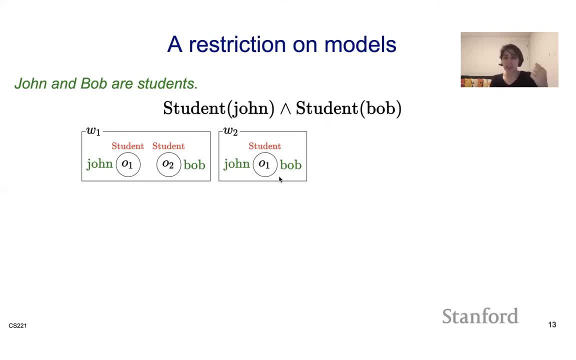 I can have a single node and I can say: well, this person's name is both John and Bob. Maybe John and Bob are the same people and we're talking about both of them being a student, So one other option is W2.. 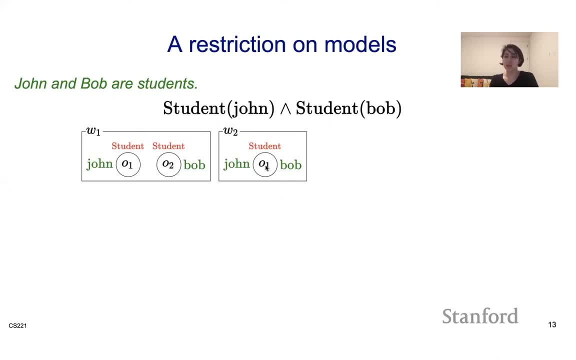 One other way of representing this model is W2, where I just write one node, Or maybe I have three nodes, Maybe I have this other unnamed node here that doesn't have anyone assigned to it. So the restriction that we are putting in here is basically trying to make sure. 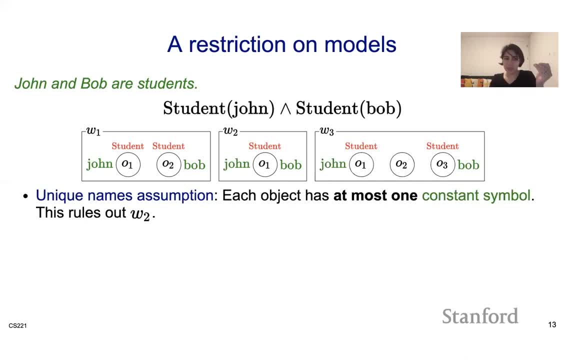 that W2 and W3 doesn't happen. So basically we are putting this unique names assumption, which says each object has at most one constant symbol for it, And this basically rules out W And in addition to W- sorry, this rules out W2.. 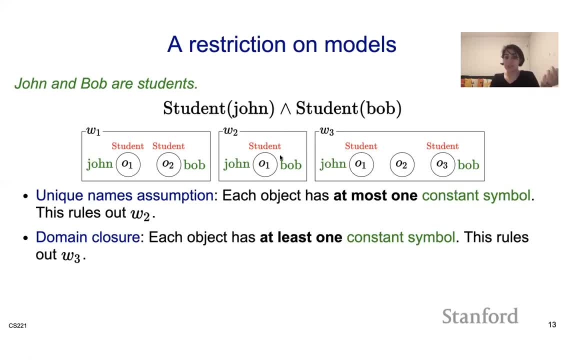 Basically we can't have both John and Bob associated to the single node, to the single object, So we can have at most one constant symbol, And in addition to that you're going to have another assumption on domain closure Which basically says each object has 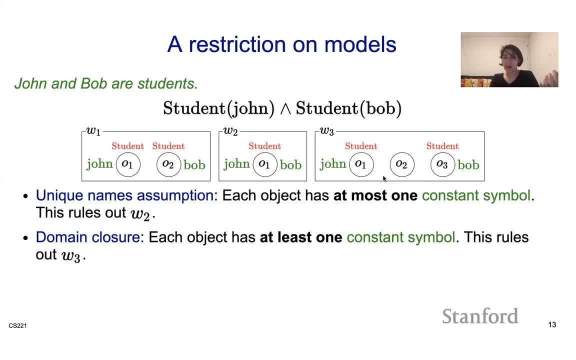 at least one constant symbol. So we can't have an object corresponding to O2 here that doesn't have any symbols assigned to it. So this rules out W3.. So this basically ensures that when we have a constant symbol, a constant symbol is equivalent to having an object. 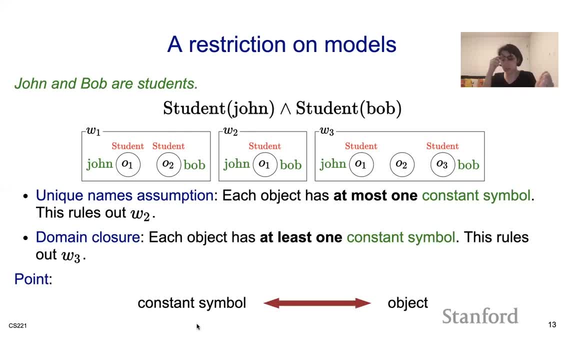 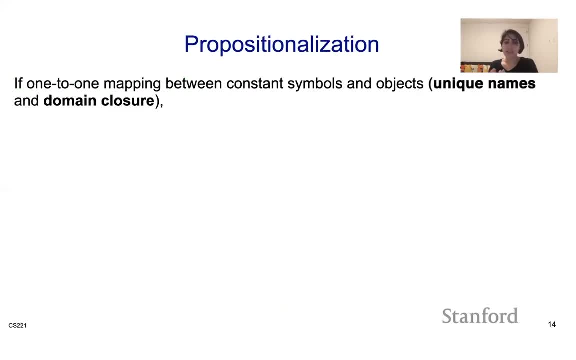 If I have an object, there is one single constant symbol that is assigned to it. So why am I trying to do this? Like what would this buy me? So the thing that this buys me, This one-to-one mapping that we have between constant symbols. 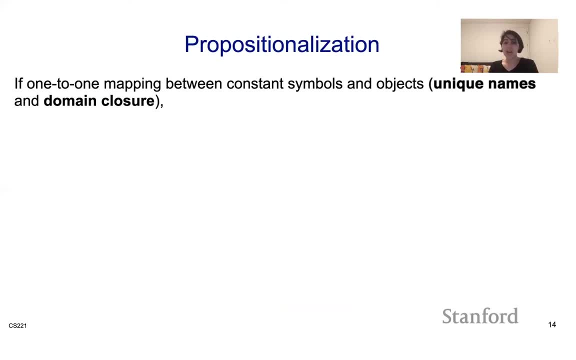 and objects like using these two assumptions that I've put allows me to do an operation that's called propositionalization, And what that buys me is actually it buys me to be able to use inference rules that bring propositional logic. The whole reason I'm doing this is: 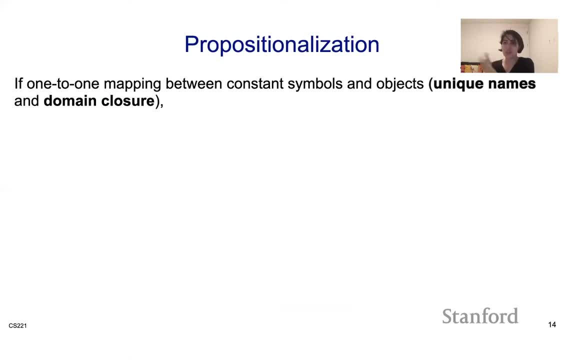 so I can use ideas from propositional logic like resolution or modus ponens when it comes to inference in first-order logic. So if you think about it, If we make this restriction, then first-order logic is not anything fancy, It's just syntactic sugar on top of propositional logic. 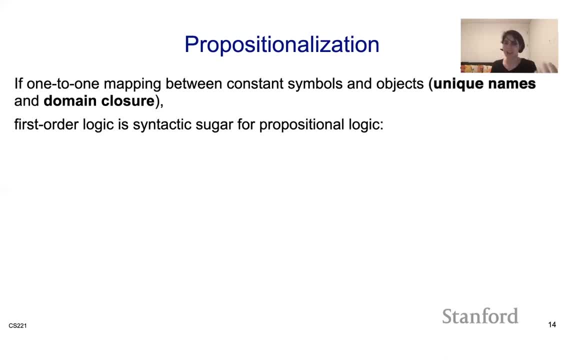 It helps us write things a little bit more expressively and have an easier time writing out things, But at the end of the day it's kind of like the same thing, the same sort of logic that goes behind everything. So, for example, if we have this example- knowledge-